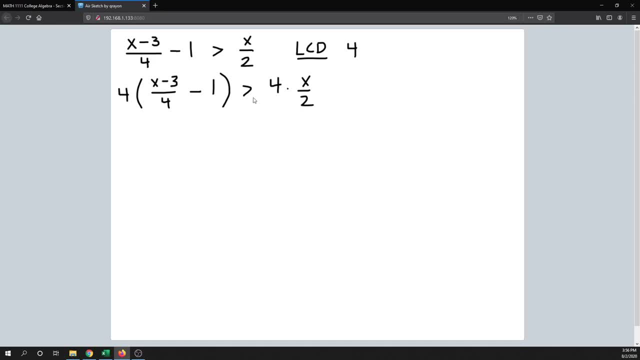 by a positive four. so there is no need to change the inequality sign. it just stays the same, All right. So next up, what we want to do is to simplify both sides as much as possible And remember, if we multiply through by the LCD, what should happen if you do it correctly. right, is that all of the fractions? 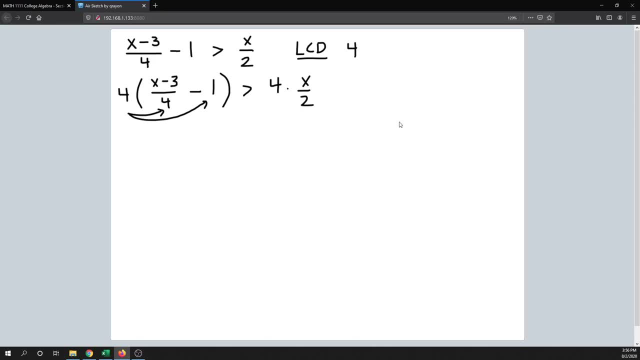 should simplify out, And so you should wind up with an equation that doesn't part in inequality, rather that doesn't have fractions in there. Okay, So the first step over here is: I am going to distribute the four, Right, So I wind up with four times. 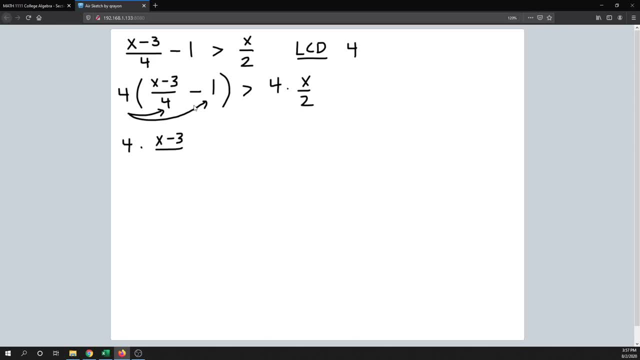 Four times X minus three over four Minus, And then four times one is four. All right, And then that is going to be greater than Over here on the right hand side. there's no need to distribute. I can just go ahead and simplify. 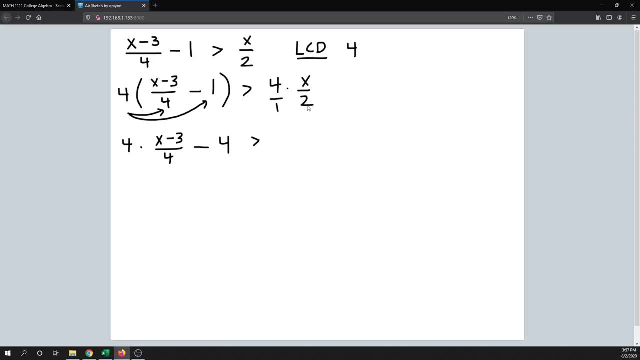 Here I have some factors on the Top and bottom with a common factor of two Right. So two goes into itself once it goes into four, two times Right. So here I have two X over one, So that's going to be a two X over on this side. 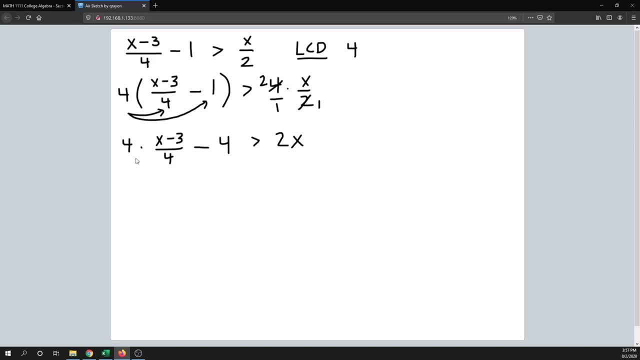 All right, Then over here, simplifying more, on the left side I've got Four on top and a four on the bottom, so I have a common factor of four. They can cancel each other Out, All right. So four goes into itself once. four goes into four once. 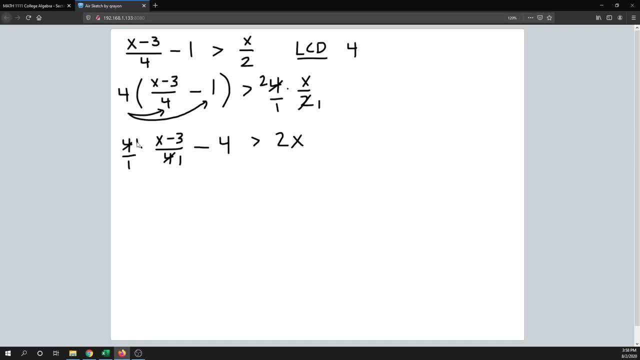 And so, multiplying these two fractions, I have X minus three times one. So on top, that's going to give me an X minus three. On the bottom, I've got A one Okay, And so One times one is one Okay. 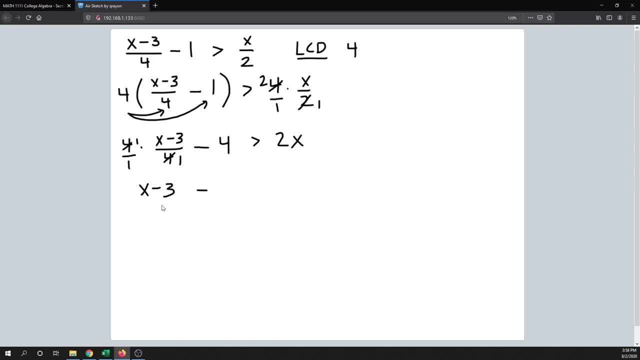 And so that's X minus three divided by one, which I'm not going to bother to write Right, Because X minus three divided by one is just X minus three. Okay, And That four tags along, And I have that less than two X there. 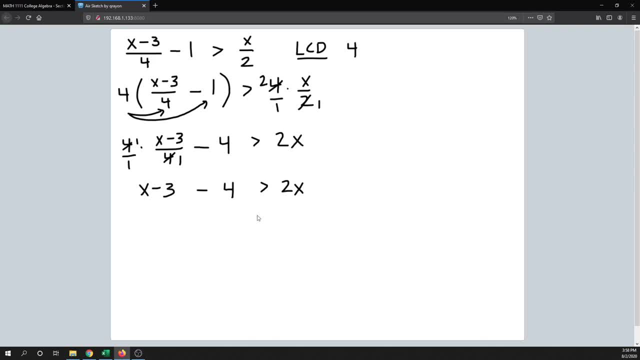 Okay, So you can see the LC multiplying both sides by. the LCD did its job. They canceled, all the fractions are gone, And so Now we would just keep simplifying both sides as much as possible. Over here on the left hand side, we have a. 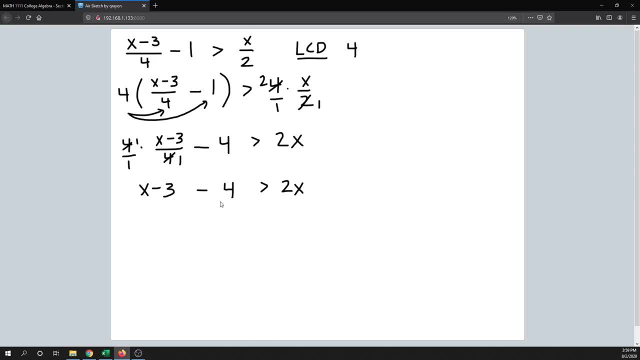 Some like terms. this minus three, minus four, It's going to give us X minus seven. And then Over on the right hand side I am going to have It already is simplified as much as possible, Right, And so I just have two X there. 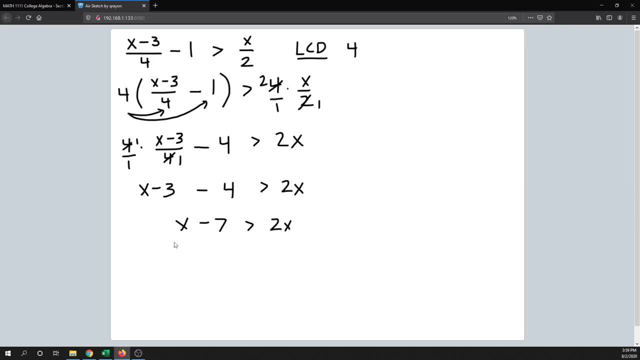 Okay, All right, So now each side is as simple as I can get it, And so then, what I would want to do is to add or subtract Right The same quantity from both sides, And remember the goal in doing that is to get every term with an X on one side. 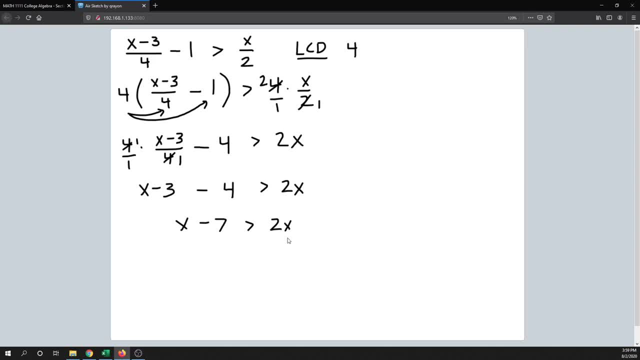 Every term without the X on the other side, And so The easiest way to do that in this particular situation Is to subtract X from both sides. So I'm going to do that. Okay, So I'm going to subtract X from both sides. 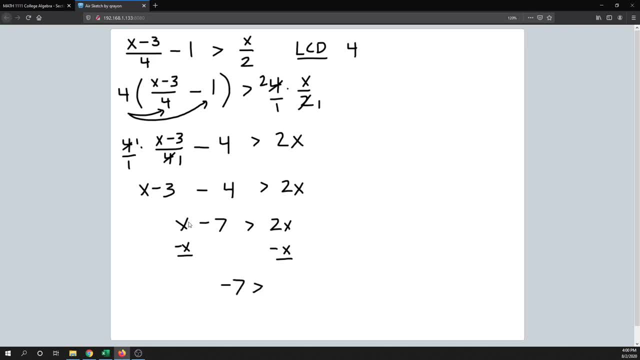 Over on the left side. I'm going to get negative seven Over on the right side. two X's minus one X Gives me X here. All right, And so then I can see there's no need to go any further. I have reached the final goal. 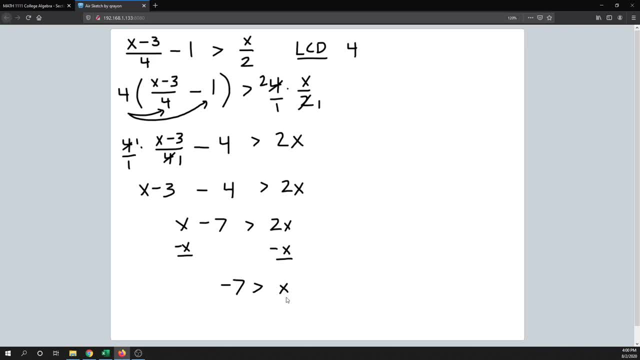 Right, Which is to get X by itself on one side of the equation, Just completely by itself, Or inequality, rather, And I've done that, Okay, All right. So What I want to do next, then, is to we know we have to graph these solutions out. 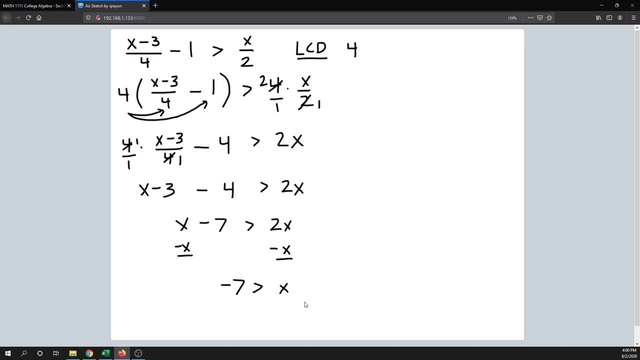 And so I am going to graph this out. And now this inequality is kind of pointing a different way than most people kind of want it, Especially if you're not used to dealing with inequalities all the time. Most people kind of want that Because some people vinegar all of that stuff. 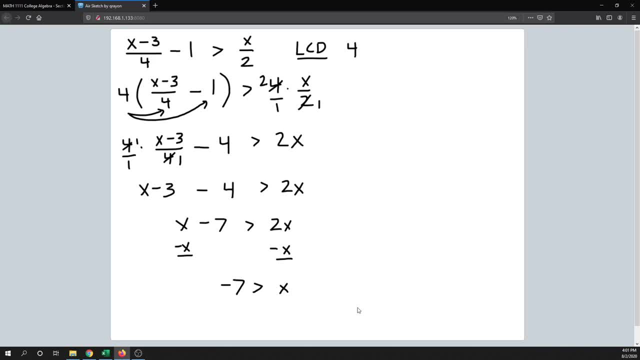 Or or whatever, it can become a little extremely powerful And that can maybe change a little bit Because of the combination of real incarnations of certain Podiums of complex flows. Okay Now, how would you get X億? Put a small section of X to represent that X to be over on the left-hand side? 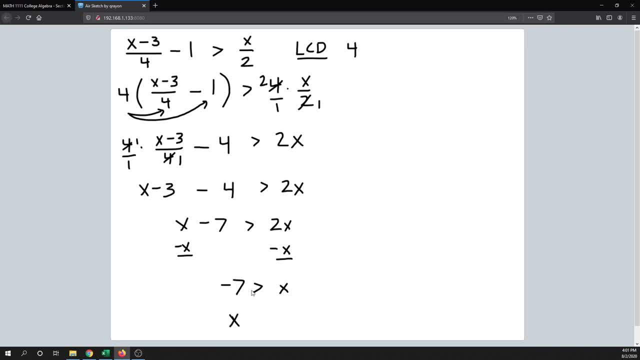 You can always write it so that the X is over on the left-hand side, If you want to. You just have to be a little bit careful about that when you do that. So if this bothers you, having this X over on the right-hand side. 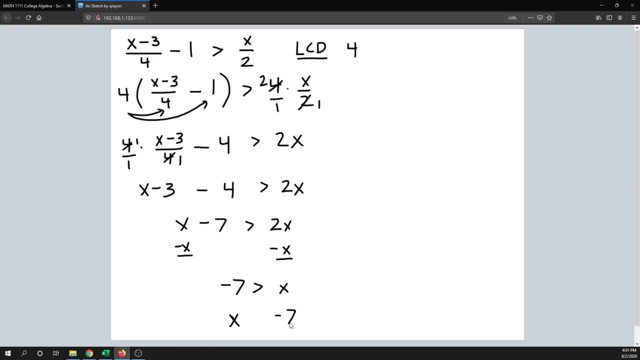 here. I took what was over on this side, wrote it over here right, and now it's a matter of getting the inequality right so that it is pointing the correct way. when you do that, so you can see that the pointy side is on the x-side. so if I 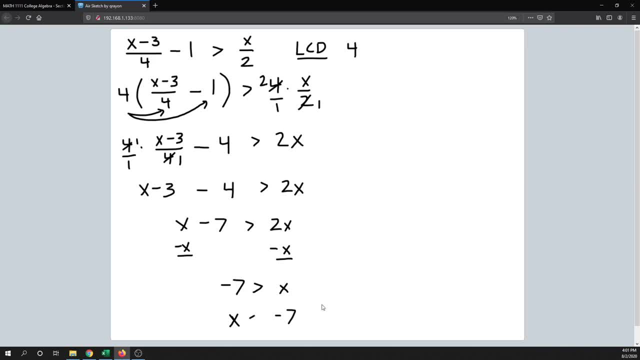 draw the inequality sign down here. the pointy side right should be over on the left side over here, and it's being a little laggy so let me refresh it all. right, the pointy side is over here on, so this is the correct way to reverse that. 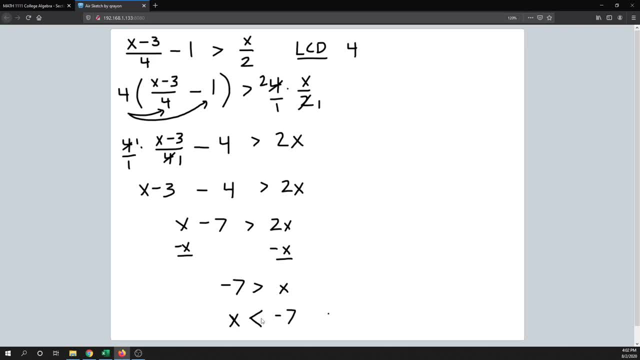 I'm not saying you have to do that, okay, but sometimes it's just easier for people to think about things when the X is over here on the left side. okay, all right. so now what we want to do is to graph this out, so I am going to go ahead. 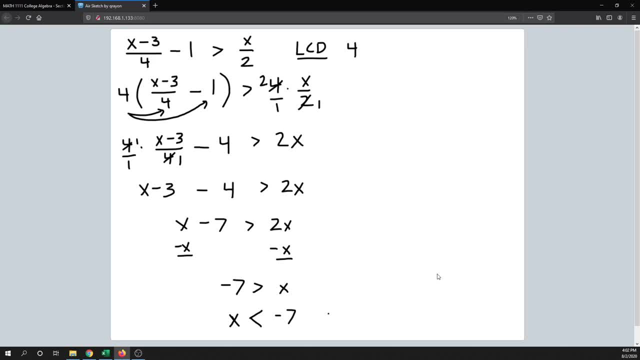 and draw my number line, and on that number line I am going to put a minus 7 in there. so here's my number line. okay, and so here, right, we can see that the solutions are to the left of negative 7. right first off, before I do that, I should note whether. 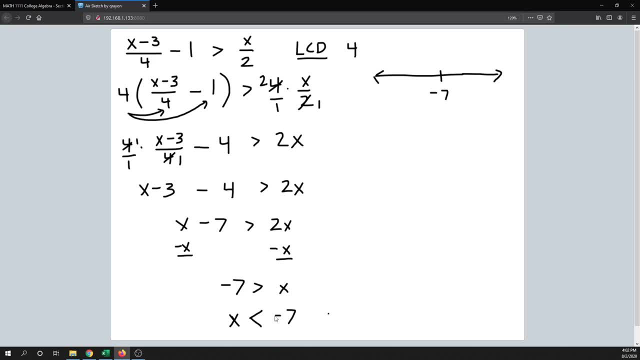 or not negative 7, will I put an open dot or a filled dot there and we can see that negative 7 is not a solution of this inequality, right? there's no or equal to there. so if I plugged in a negative 7, I'd get negative 7 is less than negative 7, which is false, right? so 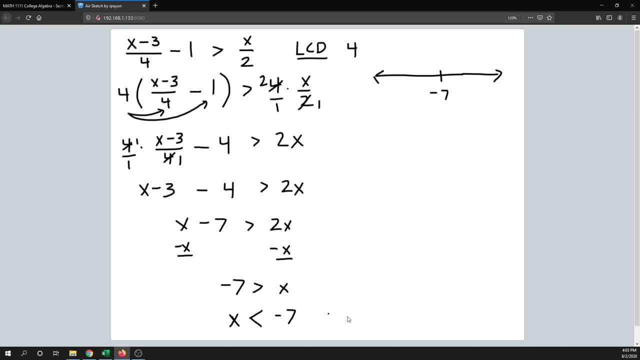 negative 7 is not a solution, and so what that means is that I should put an open dot right on the negative 7. there, there we go. there's the open dot. okay, on the negative 7, all right, and then, if you prefer to do it this way and have this on the left, you can see that the 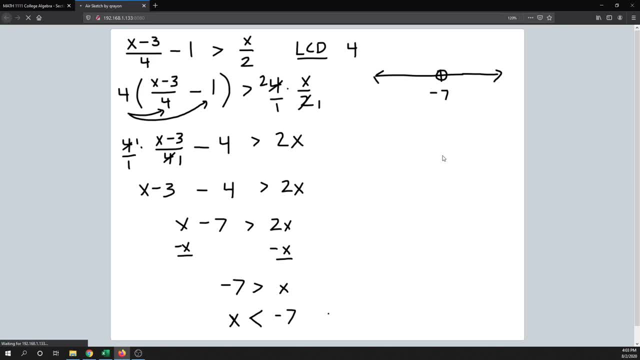 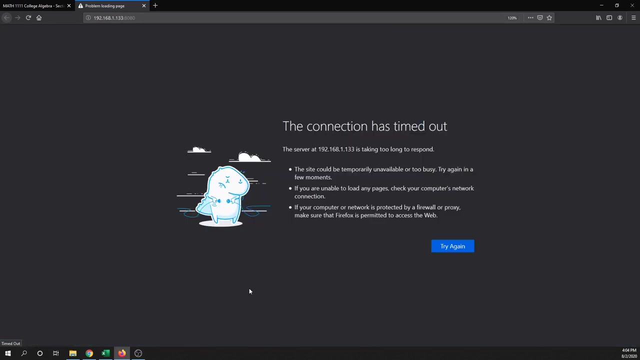 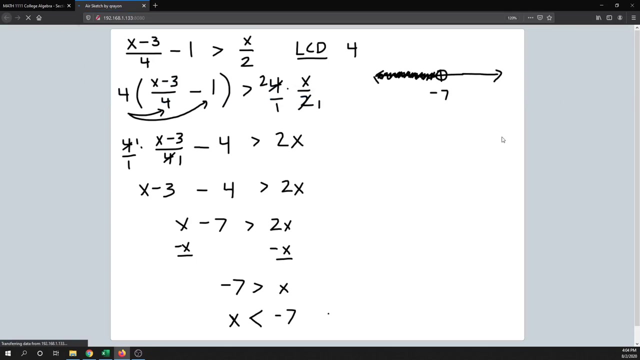 solutions X would be on the left over here. okay, so this notation kind of mimics the number line more of how the number line appears. The solutions will be over here on the left-hand side, Over on this one on the right side. Sorry, I'm having some technical problems here Over here on the left-hand side, Remember. 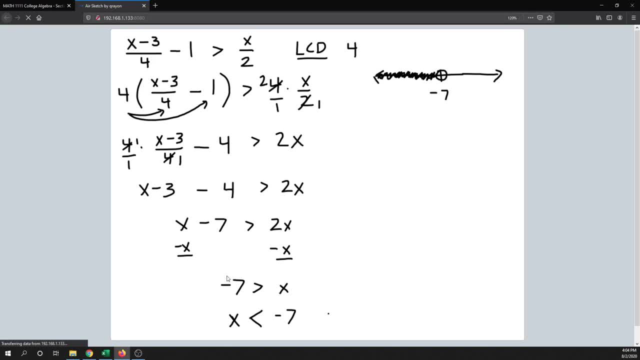 you can always decide which side to shade with these inequalities by picking a number over here. So say you didn't know should I shade the right side or the left side, Or you get confused about how to do that. You can always pick a number Like, for instance, zero right would be over here somewhere to the right of negative seven right. 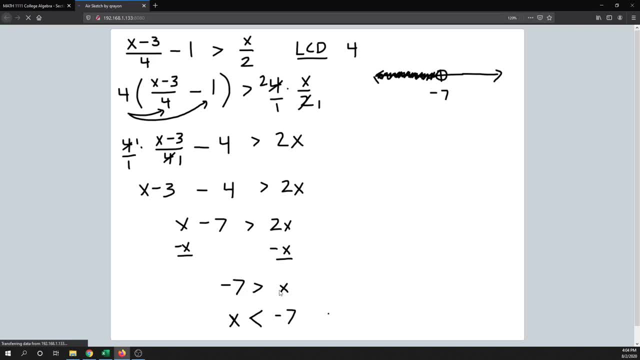 And so if I plug a zero in here, I get negative. seven is greater than zero. Well, that's not true at all. right, So that would tell you that you need to shade this other side, the side that zero is not on over here. So that's a trick that you can. 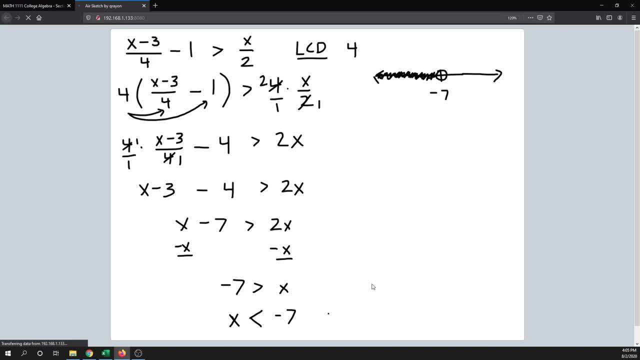 use to if you get confused about which side to shade. So you can either use that trick or the trick that I showed you about rewriting this so that the X is over here on the left side. Okay, But either way and again, those are optional things. You don't have to do anything, Just shade it correctly. So once you get it shaded correctly, then it's just a matter of writing the interval notation. The interval notation is going to look like this: right Negative seven is going to look like this: